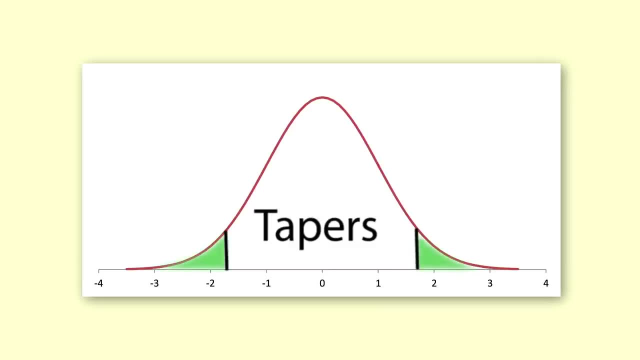 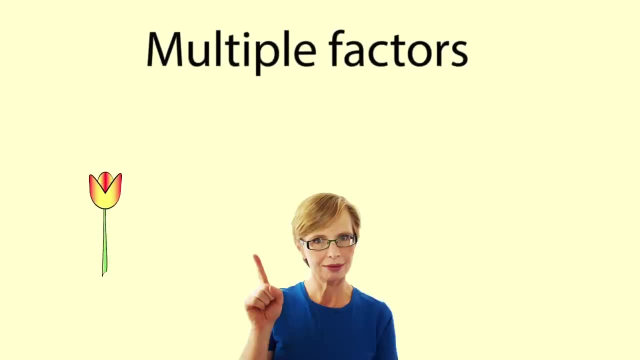 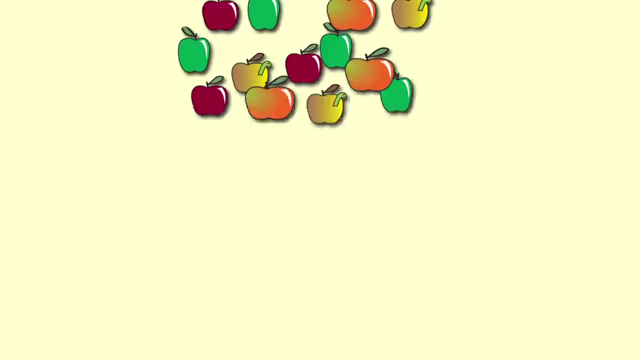 the fewer people or things occur. so the distribution tapers out in both directions, Caused by multiple factors. Whenever there are many different factors affecting an outcome, we tend to get something that is well modelled by a normal distribution. For example, if we look at the size of an apple that is affected by the sunshine, 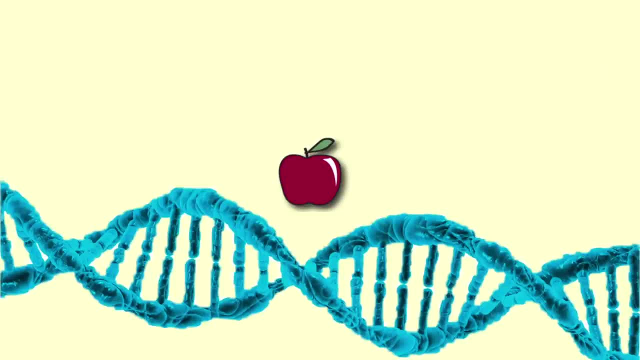 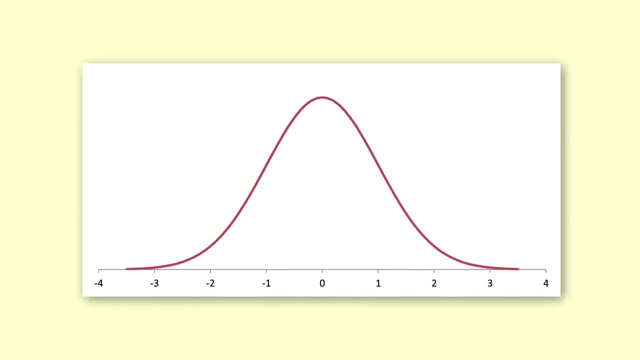 wind and rain on every day of its life. also its genetics, pollination date, fertiliser and all sorts of other things. So the distribution of the sizes of apples of the same variety would probably resemble a normal distribution. So the distribution of the sizes of apples of the same variety would probably resemble a normal distribution. 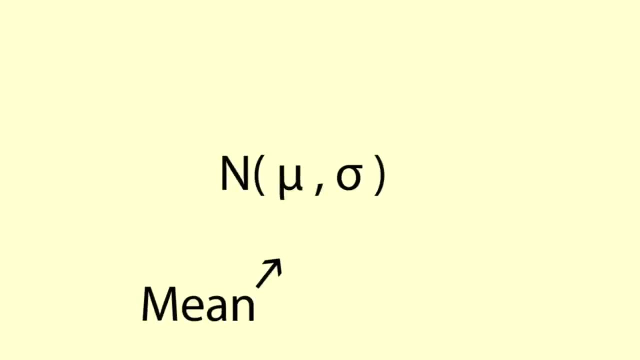 Each normal distribution is defined by the mean and the standard deviation. each normal distribution is defined by the mean and the standard deviation. The mean is also the median and also tells us the midpoint of the distribution. It is the value around which all the data values are centred. 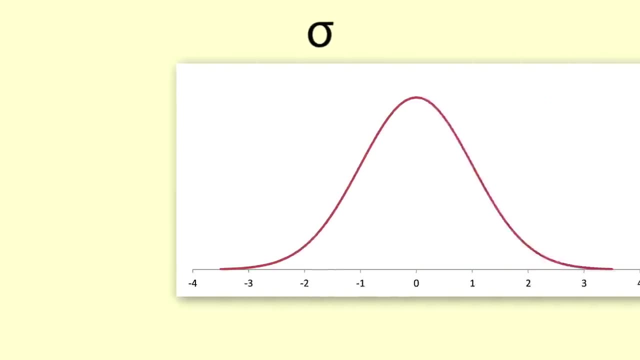 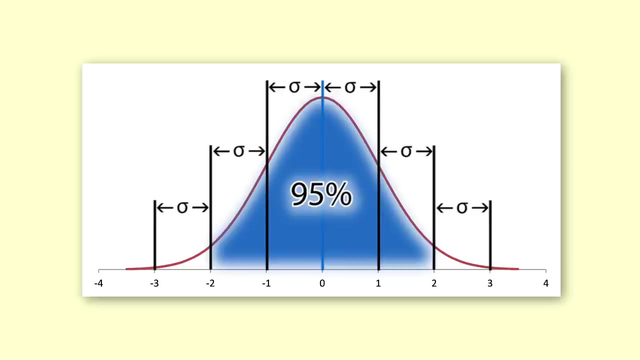 The standard deviation tells us about how spread out the data is. A useful rule of thumb is that most, or 95 % of the data values will occur within the 2 standard deviations of the mean. It is important to note that there are also many things that are not well modelled by the normal distribution. 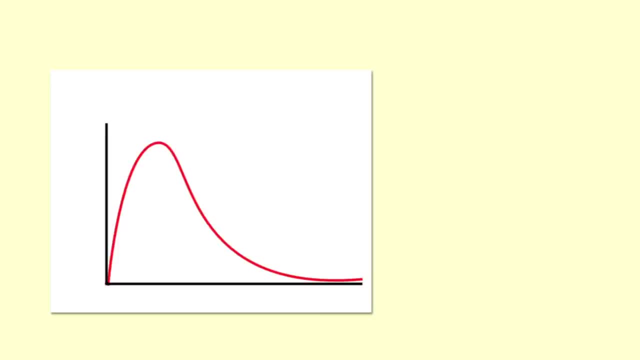 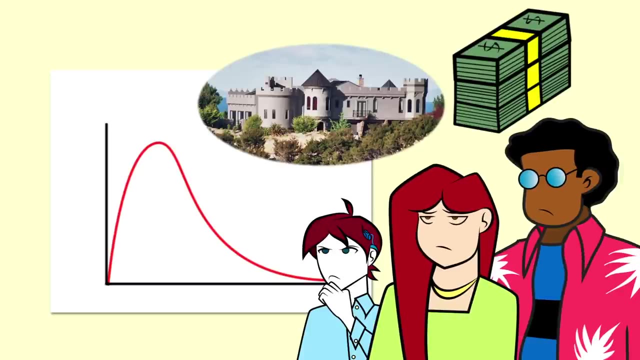 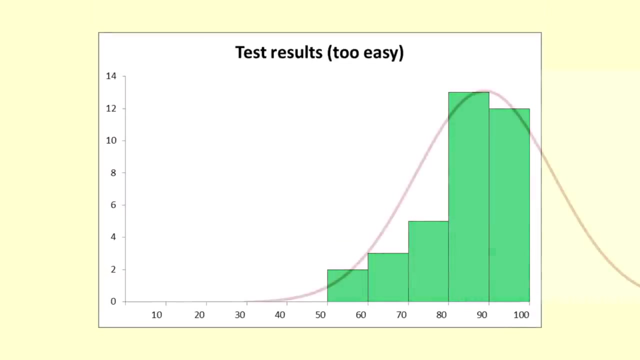 Many distributions are not symmetric and have considerable skew, often to the right. House prices, incomes and human weights are not well modelled with the normal distribution as there can be quite a long tail to the right. Even test scores in school are not always well modelled by a normal distribution. 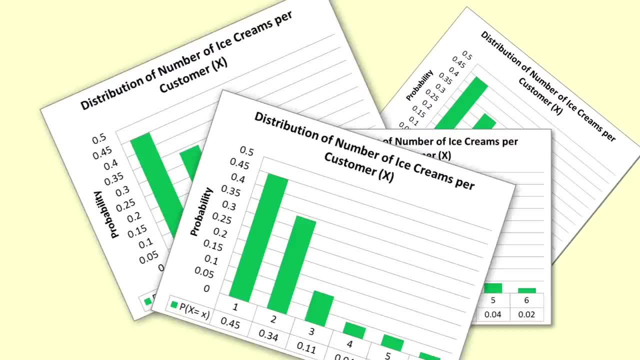 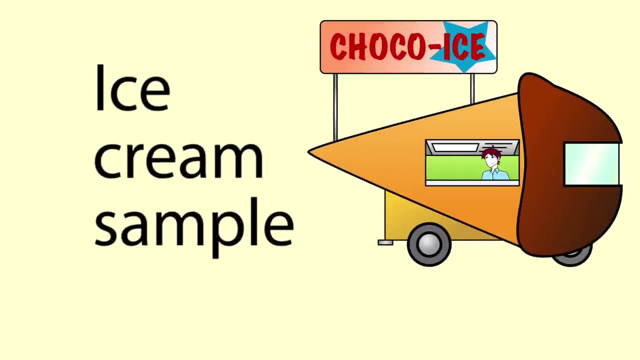 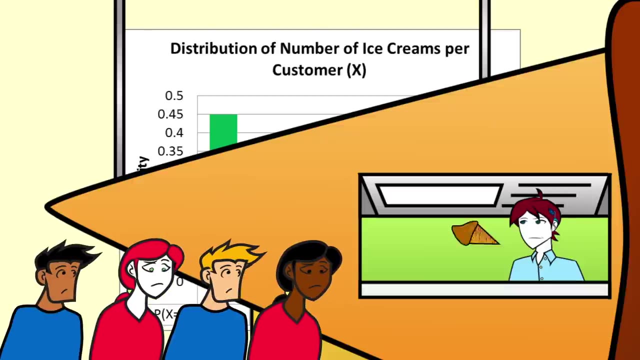 But when you add together many occurrences from even non-normal distributions, you tend to get a normal distribution pretty quickly. Here is an example of what I mean. This is the distribution of number of ice creams purchased per customer at Luke's ice cream stand. 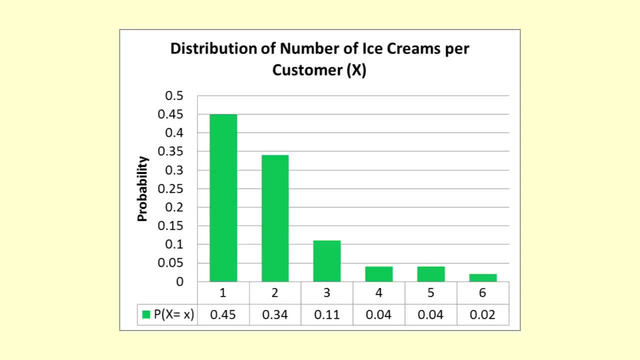 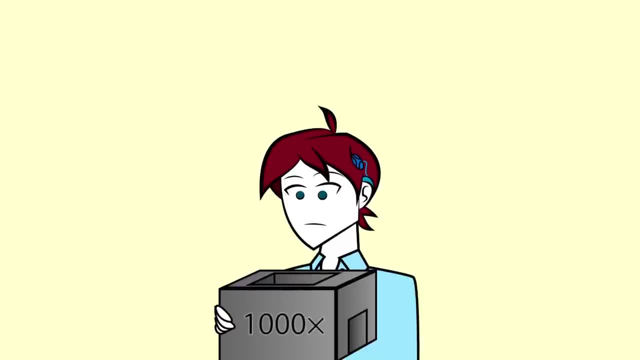 It is based on data he has collected over the last few weeks. It is clearly nothing like a normal distribution. We run a simulation of a thousand customers and see what this distribution looks like. It is similar to the original, as we would expect. 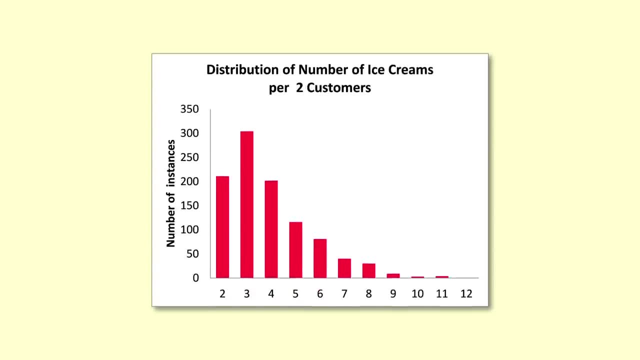 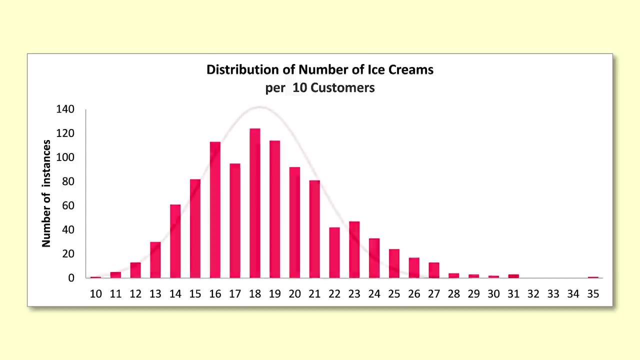 What say? we want to look at what one thousand lots of two customers buy, Or one thousand lots of three customers, Or four customers, Or ten. We see that the shape of the graph starts to look more and more like a normal distribution For ten customers to order a total of thirty or more ice creams. 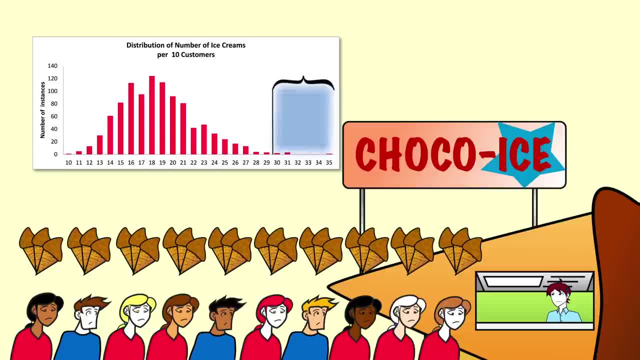 they would all need to order two or three ice creams. They would all need to order about three ice creams each, which is pretty unlikely. Similarly, it is pretty unlikely that all ten people will order just one ice cream for a total of ten. 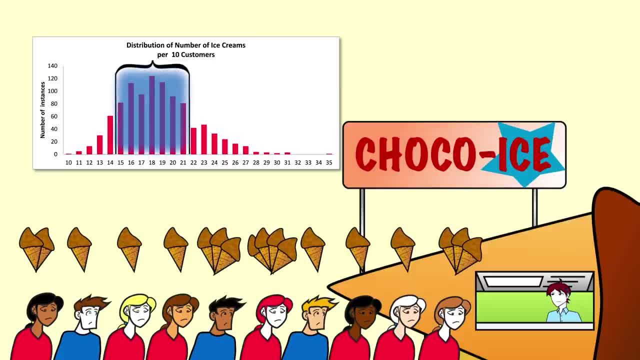 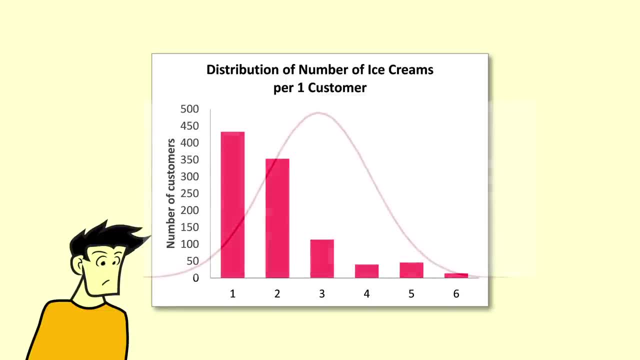 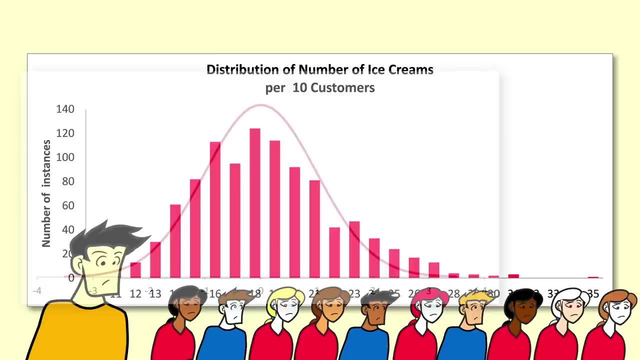 Most of the time the values will be much less extreme. So, even though the distribution for each individual customer is nothing like the normal, once we add even ten customers together, the resultant distribution closely resembles the normal distribution. That is why the normal distribution is very similar to the normal distribution. 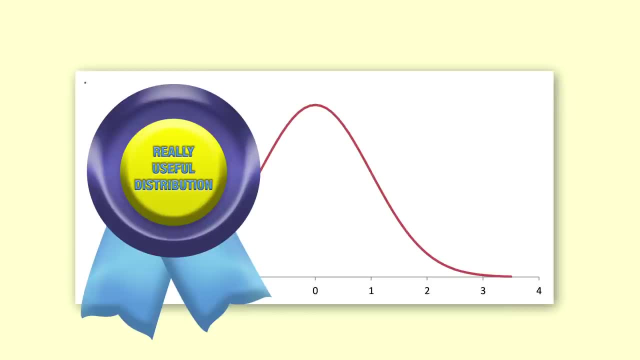 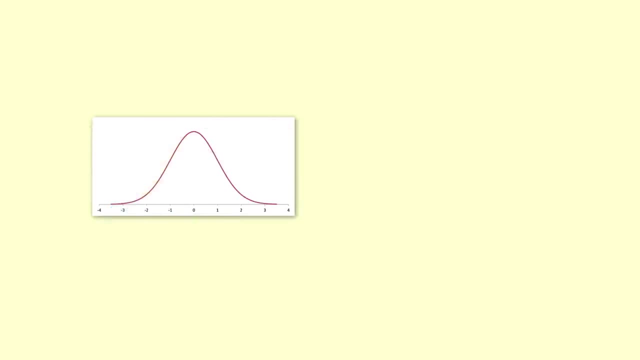 That is why the normal distribution is so useful. We have looked at the bell-shaped graph a lot in this video and now I'm going to explain how it works. That bell-shaped graph is called the PDF or probability density function, To find the probability that an outcome is within a certain range. 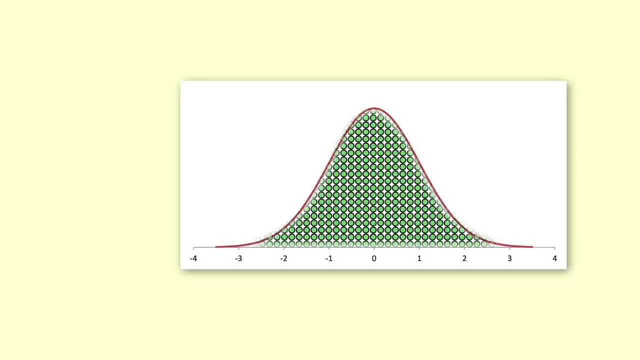 we look at the area under the graph within that range. We could think of it as the probability that a randomly chosen pixel occurs within that range. We could think of it as the probability that a randomly chosen pixel occurs within that range. Here is the PDF of a normal distribution approximating the weight of Luke's ice creams. 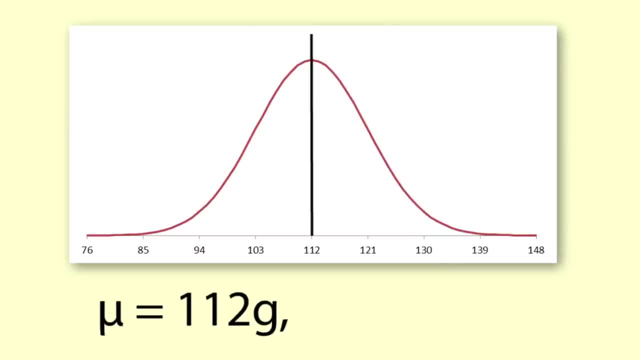 Here is the PDF of a normal distribution approximating the weight of Luke's ice creams. There is a mean of 112 grams and a standard deviation of 9 grams. There is a mean of 112 grams and a standard deviation of 9 grams. 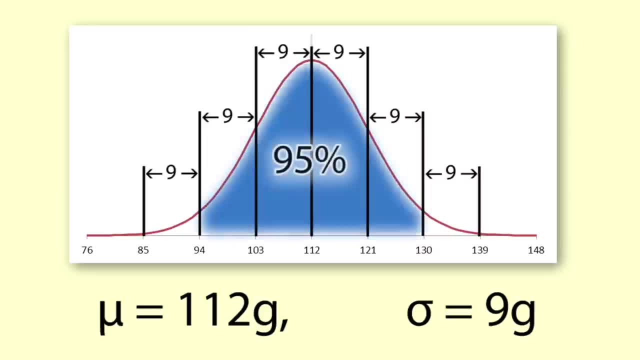 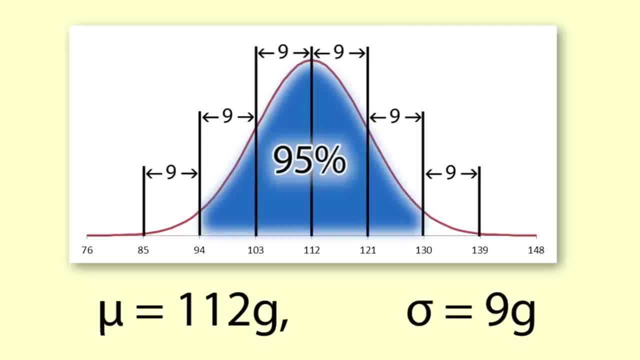 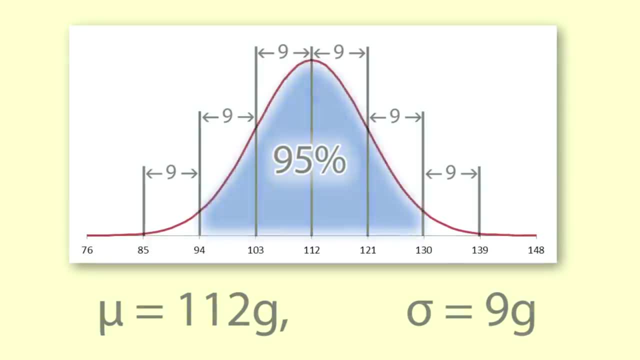 This is always true for normal distributions. This is always true for normal distributions. So we say that 95%, or most ice creams weigh between 112-18, which is 94 grams, and 112-18, which is 130 grams. You can see that 95%.